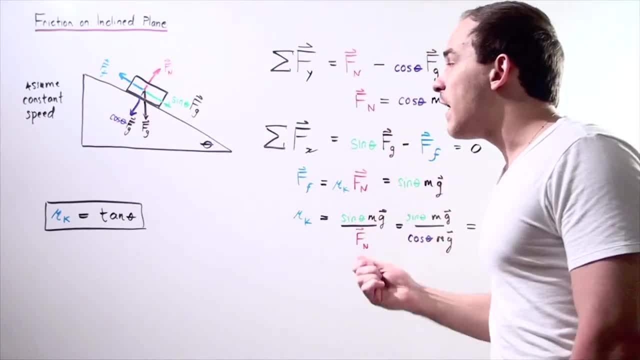 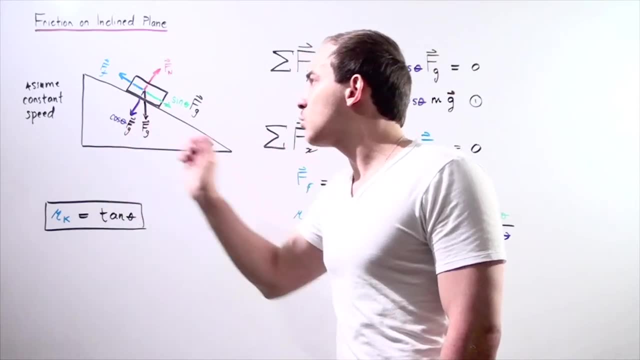 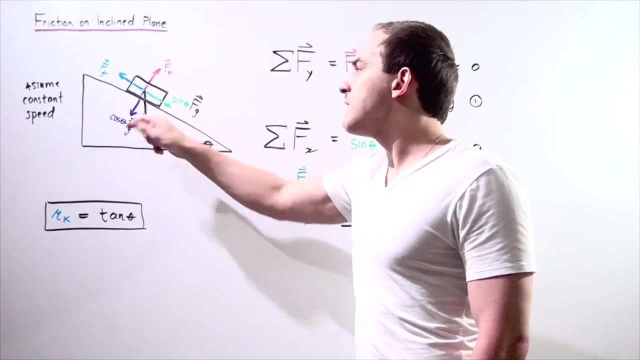 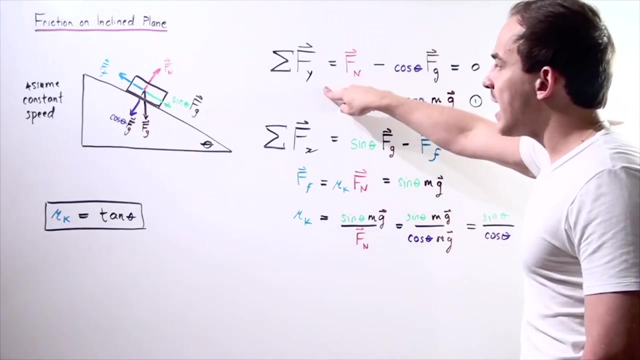 In the negative direction along the x axis. And finally, there is also a component force that acts in the negative direction, runs in the negative direction of the y axis shown here. So the cosine of the angle multiplied by the magnitude of our gravitational force. So now let's sum up all the forces acting along the y axis and all the forces acting along the x axis. 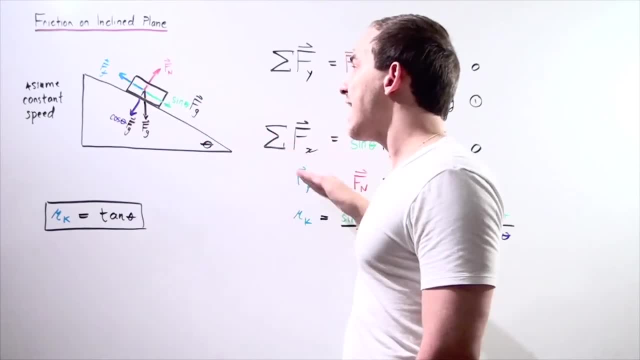 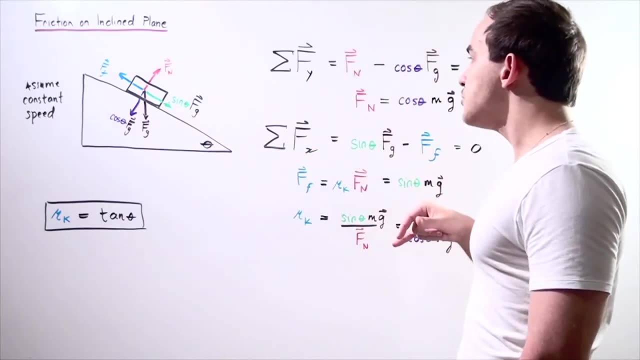 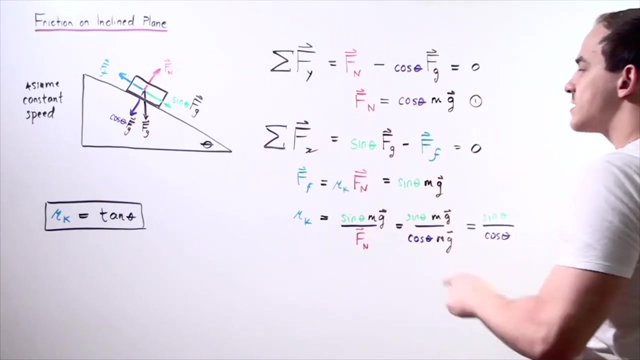 Now, because we have constant velocity along the x axis and because our object is not moving along the y axis, both of these summations will be zero. We set them equal to zero. So let's sum up all the forces acting along our y axis We choose: going upward to be positive, downward to be negative. We have the normal force minus the cosine of the angle. theta times the gravitational force equals zero. 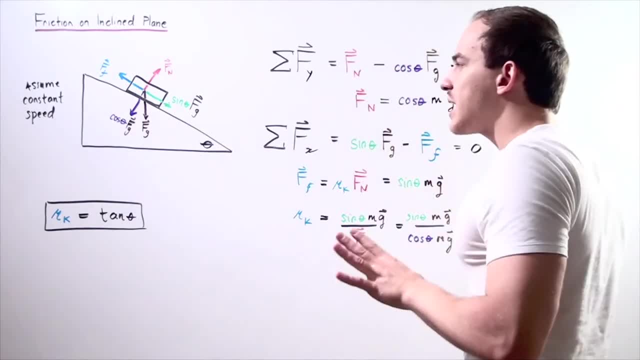 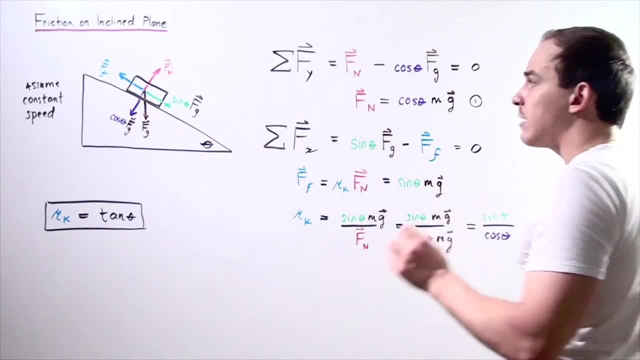 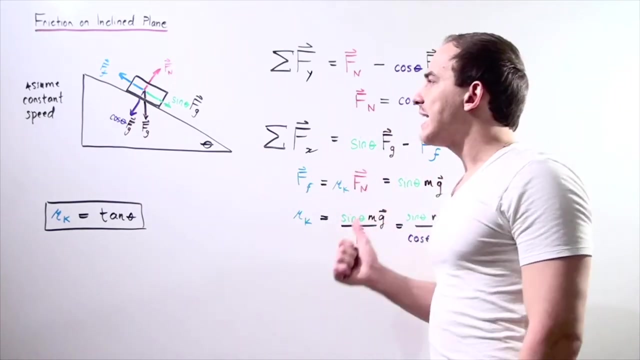 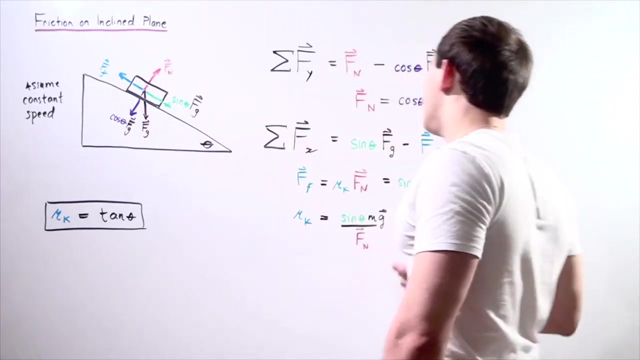 éra, this guy to the right side, and we see that our normal force is equal to the cosine of the angle theta x, the magnitude of our gravitational pull. So mass times, g. Now let's sum up all the forces acting along our x axis. So therefore, we choose, going this way to be positive and going back up to be negative. 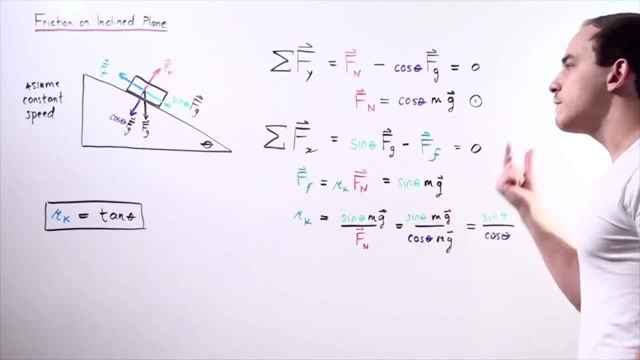 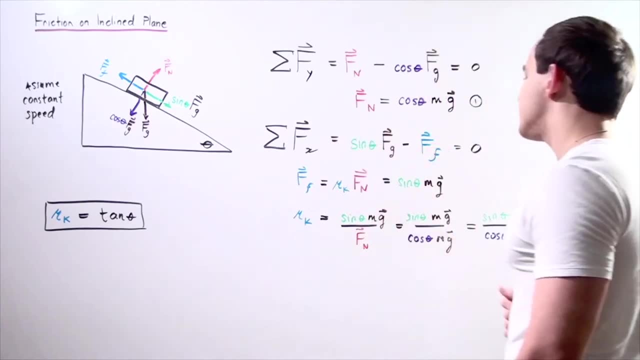 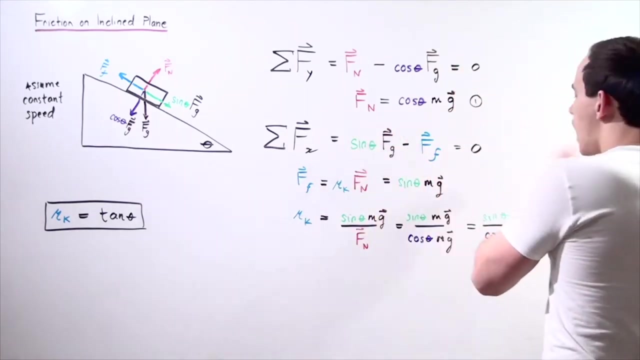 We have sine of the angle theta x, the magnitude of the angle theta multiplied by terrace얼 Minus, the force of friction equals zero because once again, we have no acceleration, We have constant velocity, constant speed. So let's rearrange, Let's bring the force of friction to one side and this guy to the other side. 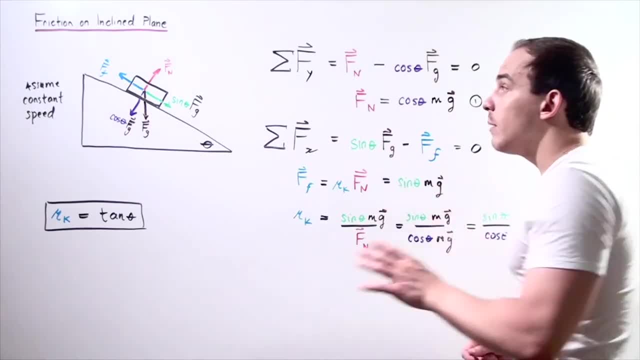 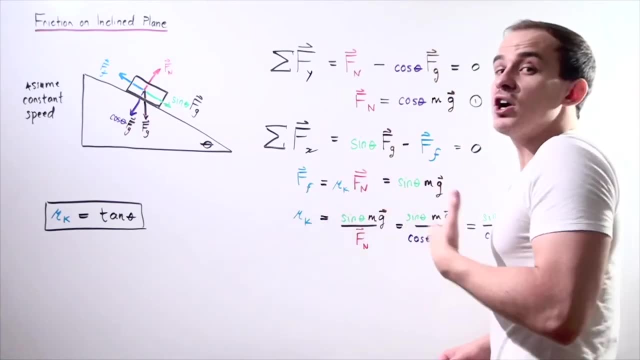 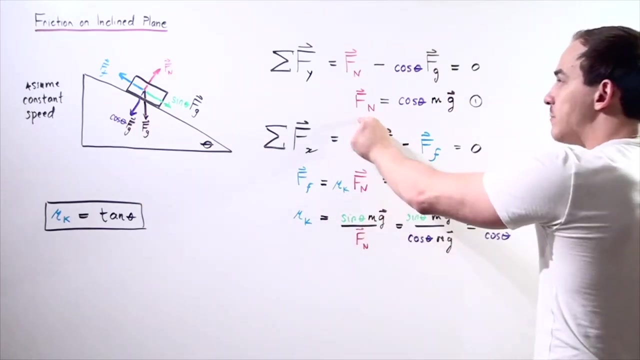 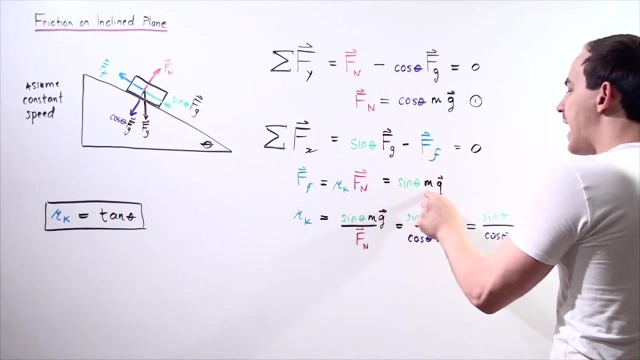 So force of friction, which is equal to well, because our object is sliding, it's moving, we're dealing with kinetic friction, So this equals to the coefficient of kinetic friction multiplied by the normal force. So we represent it with the same color as before because it's the same exact normal force. Equals sine of the angle theta multiplied by m times g, where m times g is simply our force due to gravity.